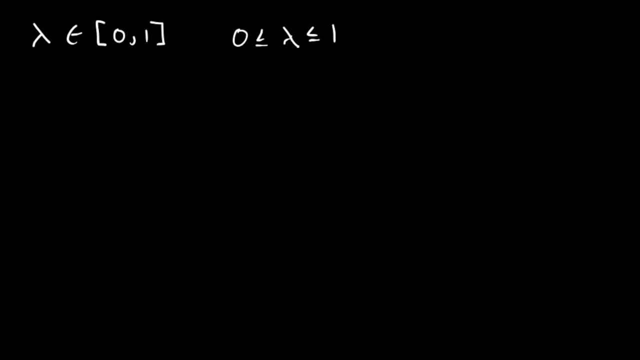 equal to 0 and is less than or equal to 1.. So at the moment this is going to be, at the moment, this is just some random variable with not much meaning, and what we're going to do now is define what a convex set is using lambda. So let's just 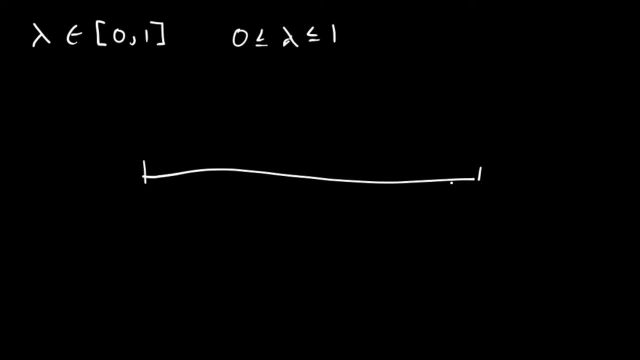 imagine a number line for a moment. That's a terrible line. Let me just make this line a little straighter. So let's just imagine a straight line, reasonably straight line, and we're going to define lambda. So let's just imagine a straight line, reasonably straight line, and we're going to define lambda. Now you might say: why is this a straight line? 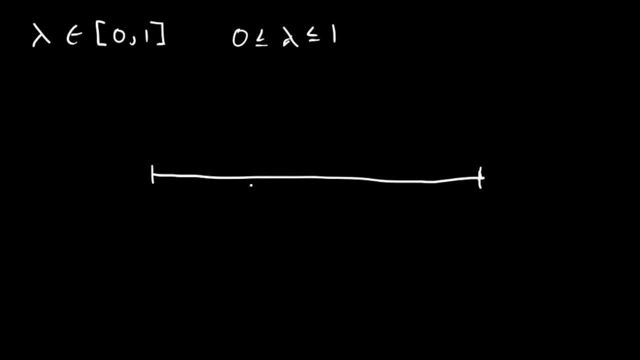 sounds better. that is say, we have two variables on this line: x, which is say 2, and then we have y over here. Let's say y equals 4.. And this is just a line of numbers. let's: 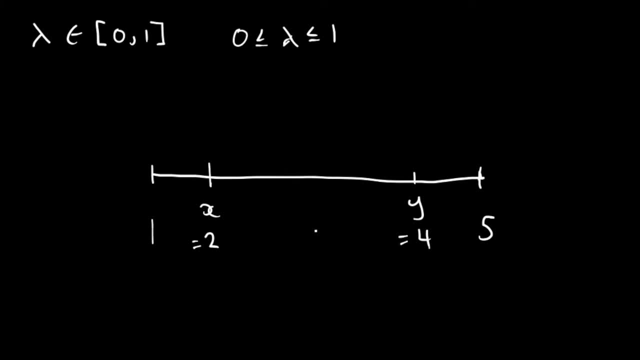 say: 1 is over here, 5 ends over here. this is just a set. What we want to do now is take something called the linear combination of these two points, of any two points contained in any set here. This is our set. say, the number line, this is our entire set. Any linear. 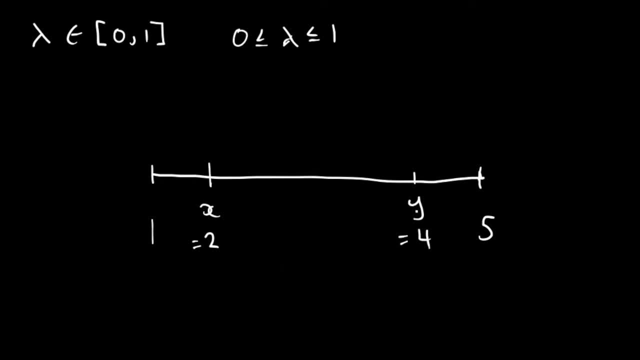 combination of any two points within the set. so point y, point x is going to be the following: So we take lambda, we multiply it by x, and we plus 1 minus lambda and multiply it by y. This is what we mean by the linear combination of any two points within a set. So let's say: 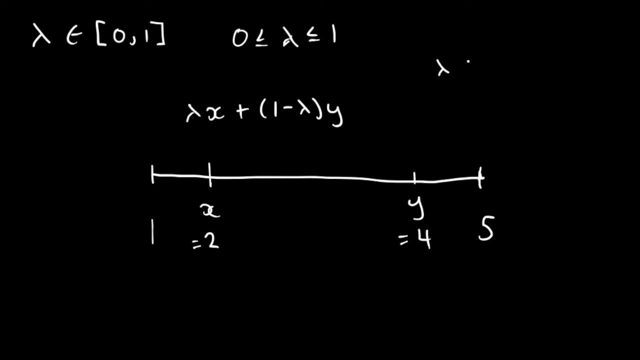 in this case, let's set lambda equal to 0.2.. What this is going to mean is that the linear combination of these two things, when we plug in x, equals 2, we're going to have 0.2 multiplied by 2.. 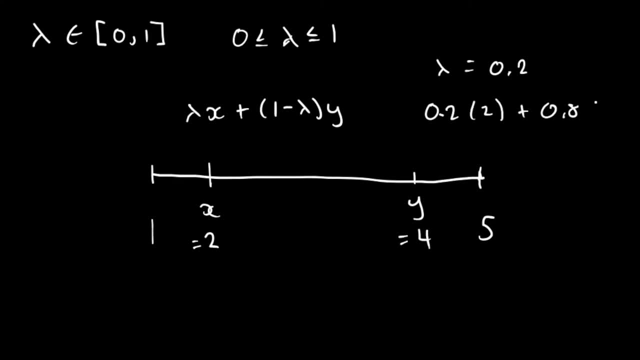 Plus 1.8 multiplied by 4,, which means our linear combination with these values of lambda equaling 0.2,, y equaling 4, x equaling 2, our linear combination is going to equal, I think, 3.6,, which is what happens when you just plug in all these numbers into this right. 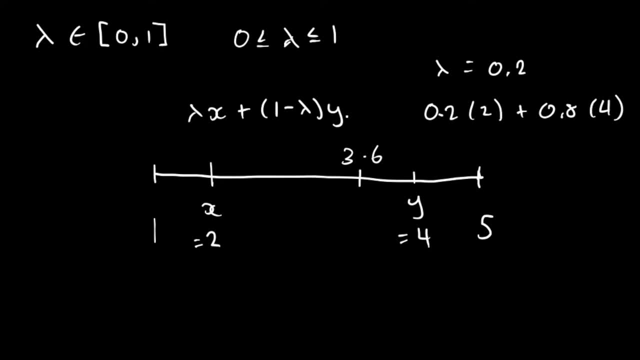 here. So what does that mean? What was the point of that? What this is doing is: it doesn't matter. we can pick any lambda, as long as it's in between, it's contained within this interval here, which is why we kind of laid out this. 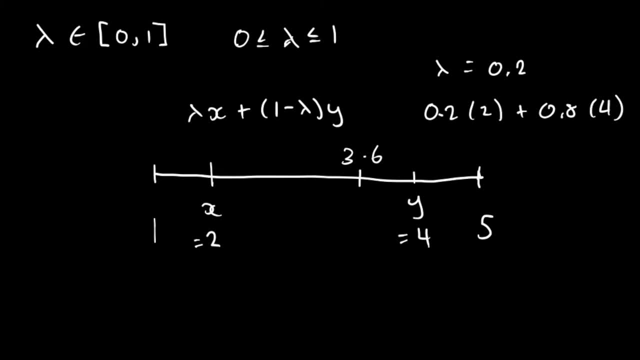 definition to begin with, As long as lambda is in between or equal to these two upper and lower bounds in between 0 and 1, any number that we plug in is going to be somewhere in between these two points. What I'm going to quickly do now is kind of draw this in a different way in a set. 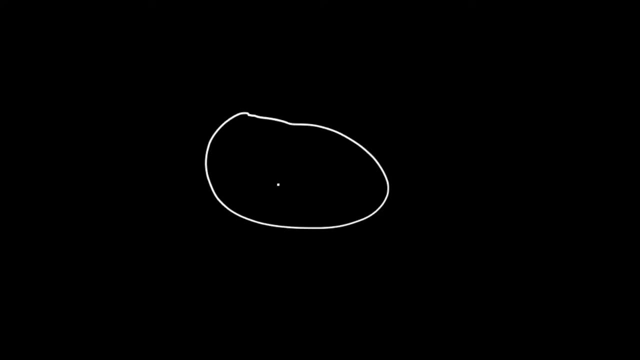 So let's say we have- this is our set. instead of being a number line, it's a circle and we have two points, x and y. again picking two points in the set, We can pick any lambda and as long as lambda is any number between 0 and 1, or equal to 1 or equal to 0, convex. 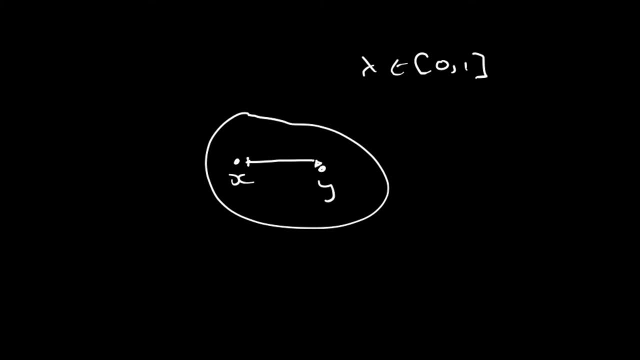 set. That means that we can draw a line between these two points. We can draw a straight line between two points in a set, x and y. And that's what the linear combination, which once again I'll draw over here. that's what the linear combination is. It's basically: 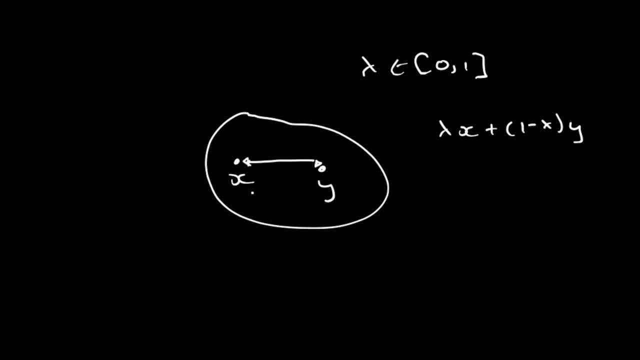 just drawing a straight line in between these two points, any two points in a set. So an example of a set that is not convex is, say that we had some sort of weird set of numbers that looked kind of like this. if you were to draw them like a set that looked like this: This is the space and you 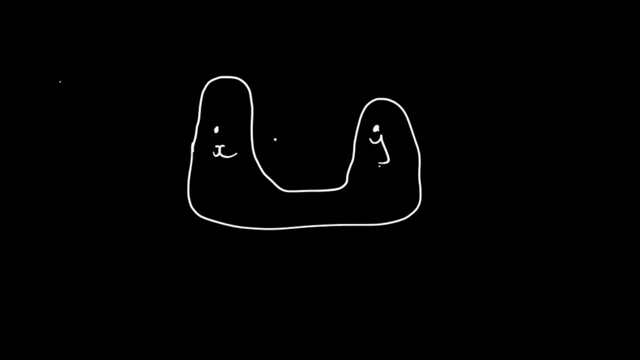 had two points here x and another point here y. As we can see now, when we have a line connecting these two points, that should be straight. when we have a straight line connecting these two points, the members, the containing two members of the set. it's not contained. 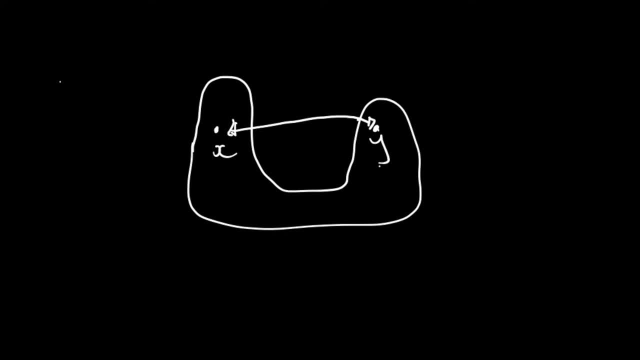 within the set is not contained within the set entirely, which means the set is not convex. So, going back to this example, because this set here contains the line segment between two of its members, x and y, these two members of the set, because it 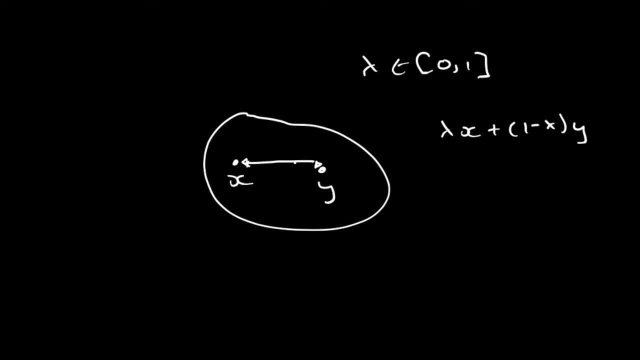 contains its entire line segment, it is convex, whereas this set is not convex because it doesn't contain the entire line segment. as you can see, it dips out of the set here, Whereas in the number line example, as you can see, this entire set here, 1 to 5, is the entire set. we can pick any linear combination and it will. 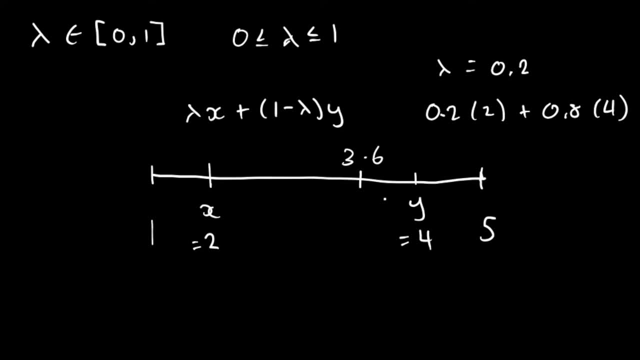 all be contained within the set 1 to 5. still so that is a convex set. So now, knowing what we know about a convex set and linear combination of two points within a set, let's use that knowledge to look at a simple function that we're going to draw on, a simple 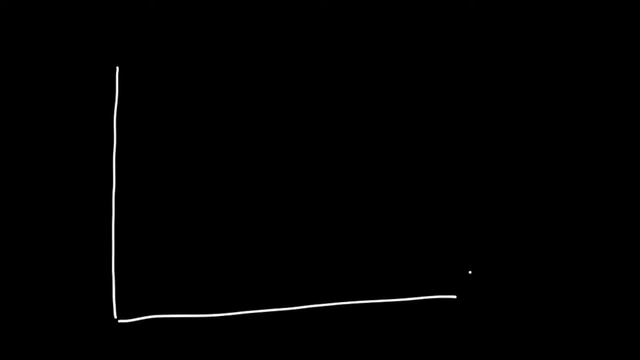 two-dimensional graph with our x-axis here and our y-axis here. So let's say, on the x-axis, let's pick two points here, point x and point y. So these again are two points contained within our set, with the set being the x-axis and the y-axis. 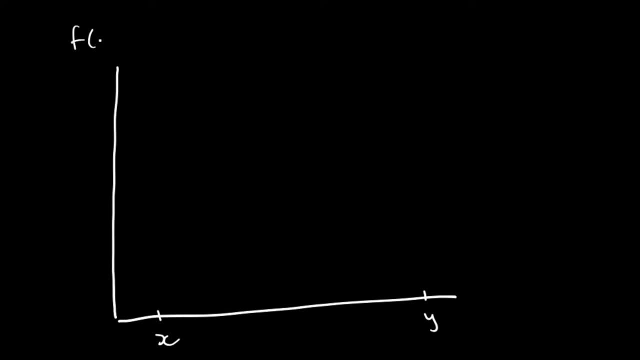 Now let's say our y-axis is some sort of function that maps these points here into the y-axis and let's say the function looks something like this, This kind of curved shape. let's map our points on the x-axis to the y-axis. 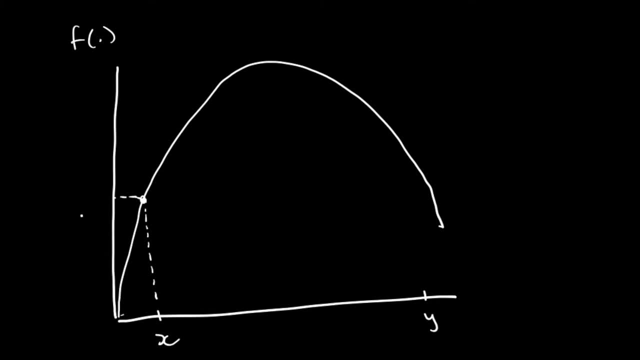 based on the shape of this function. So that's what the f of x is going to be. Let's say we have y over here. Let's make this straight as we can. This is where f of y is going to end up. So we have two points on the x-axis and 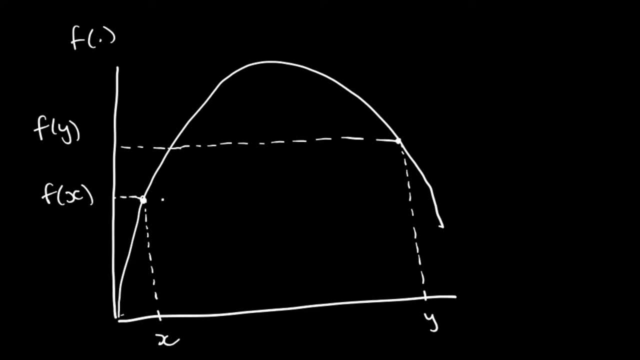 we have a function which is going to kind of dictate where these two points in the x-axis get mapped to on the y-axis. So there's our function of y, which is where y meets, the function, our function of x here, which is where x meets. 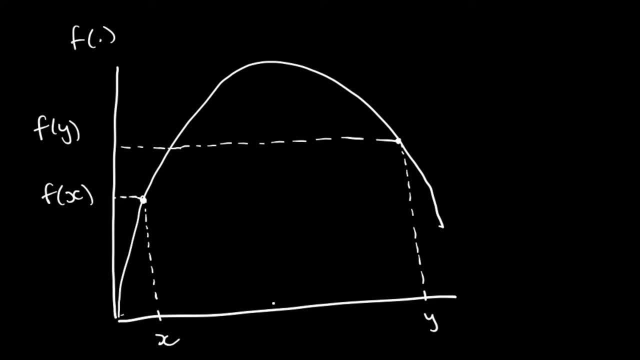 the function. So now let's start by taking the linear combination between x and y, which, as we know, is going to be this. Let's write it out once more And let's just call this now L, just so we don't have to write this out every time. 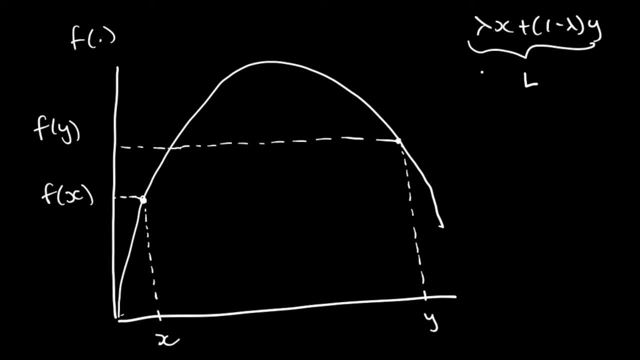 Let's call this L. So let's put L. Let's pick any lambda. Remember now at lambda, Go on running L. So that's lambda, which is just again. I've written this about three times. it's just going to be contained within the interval 0, 1.. Let's take a. 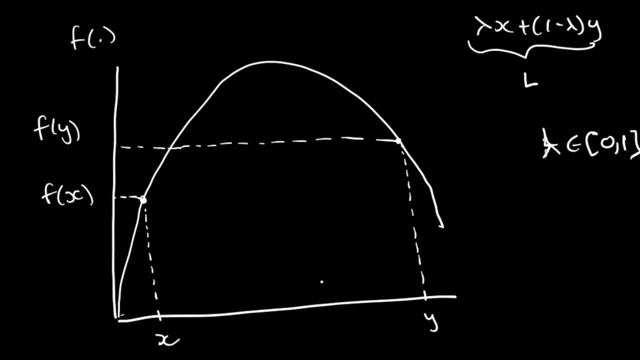 linear combination between x and y which, as we know, is going to end up between the two points. So let's say, right here, smack bang in the middle, We take our linear combination. Let's now map our linear combination to the function that we've just drawn. Now this over here goes to: 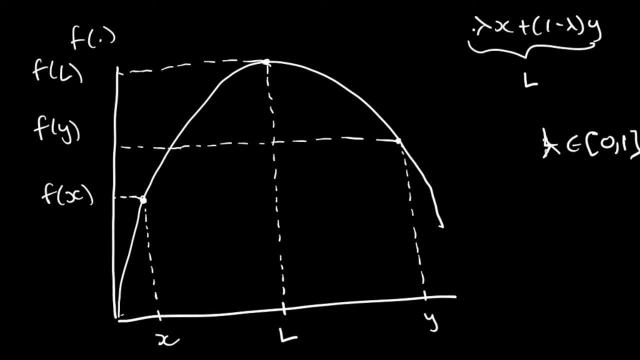 be L, So the function of the linear combination. So I'll just write this out in, I'll elaborate on that. So that's what. That's what this is. here We've taken a linear combination of two points on the x-axis and we've mapped them in the 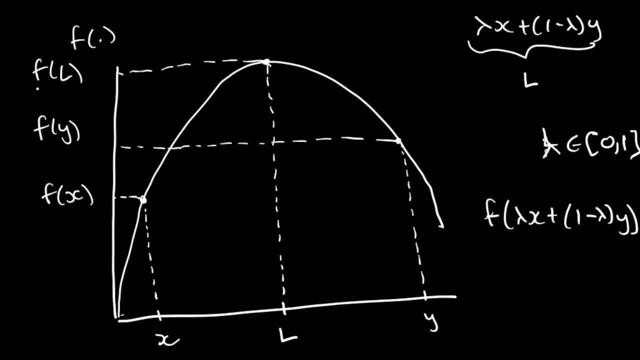 function. So this is what this is here. These two things are identical. So now what we're going to do is again take the linear combination of two points on this graph, but this time we're not going to take the linear combination of x and y on our x-axis. 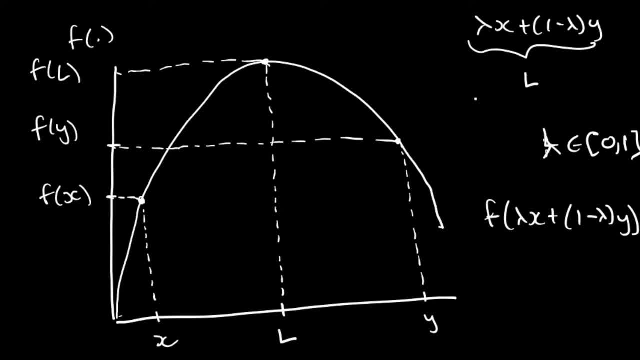 because we've already got that here, which we've just called L, and we've got the function of that over here, which we've just called f. Now we're going to take the linear combination of these two points, the function of x and the function of y. 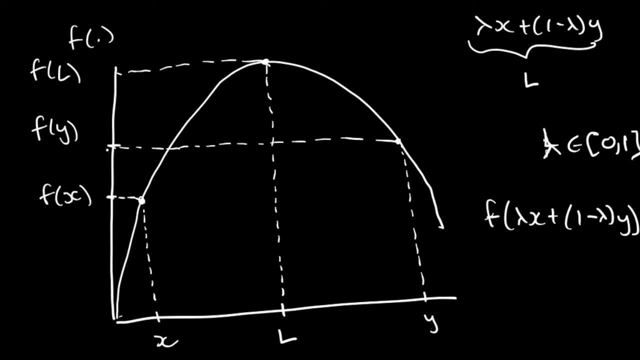 If we take the linear combination of these two points, we're going to get some point again that's going to be contained within the two, So let's again take some lambda. that means that we end up nicely in the middle between the two points, And this is going to be. I have to write this a little smaller, sorry if it's hard to see. 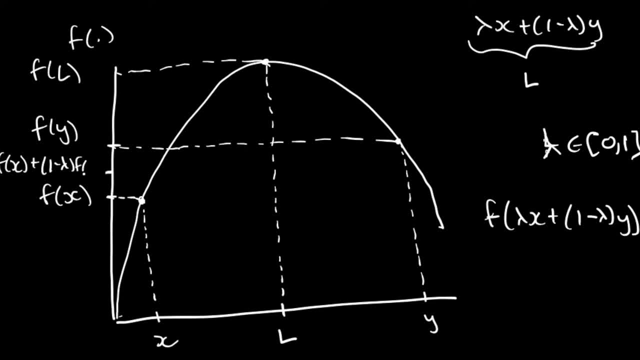 This is going to be the linear combination of the functions. I'll write this out here so it's a little bit clearer. This is going to be the linear combination of f and f. Okay, So this is going to be the linear combination of f and f. 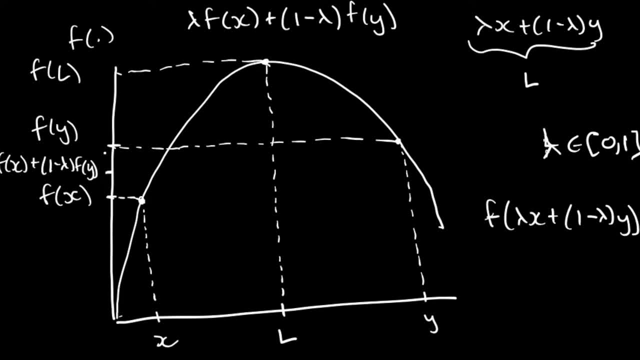 So this is going to be the linear combination of f and f, Which is going to end up in between the two points. So now we have two key things that we're going to kind of you guys are going to need to understand in order to know what we mean by, say, a concave function, which would then lead 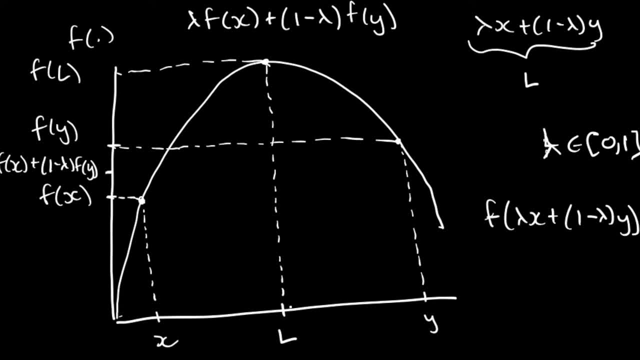 us to a convex function Is: we've got the function of the linear combinations, f, which is this here, and we've got the linear combination of the functions, which is going to be in between the two functions. And again, the first one was in between the two points and now the second one is in between. 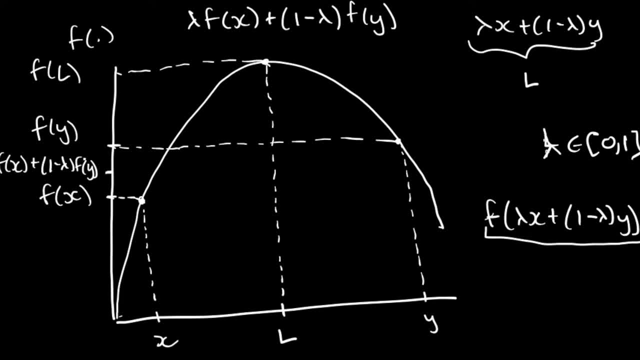 the two functions. because, remember now, when we take a linear combination with lambda e being contained within zero or one, it always ends up between our two points that we're looking at. So, the linear combination, what we're going to do is we're going to draw just another. 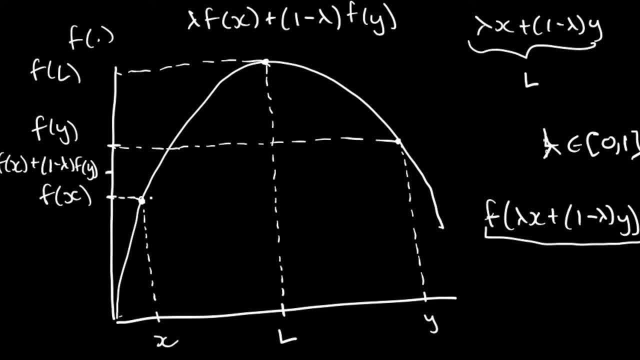 line. I'm not going to draw any more. I'm going to draw more lines after this, before it gets a bit too confusing. but I'm just going to draw another line here. It's going to be a nice straight line from point x to point y. 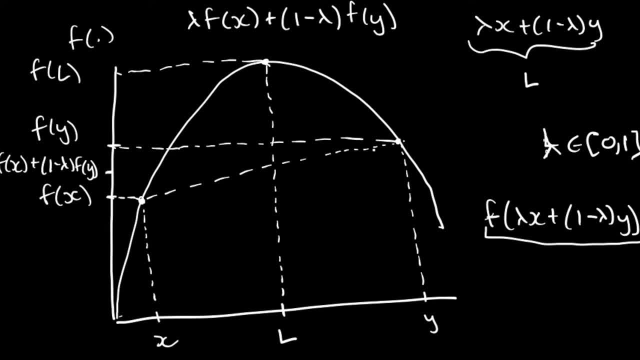 This is our line. that is going to be the linear combination of the functions. So let's say, this one ends up right here. If we picked another linear combination, let's say here, it would be there. That's what this dotted line across here represents, is when we take the linear combination of: 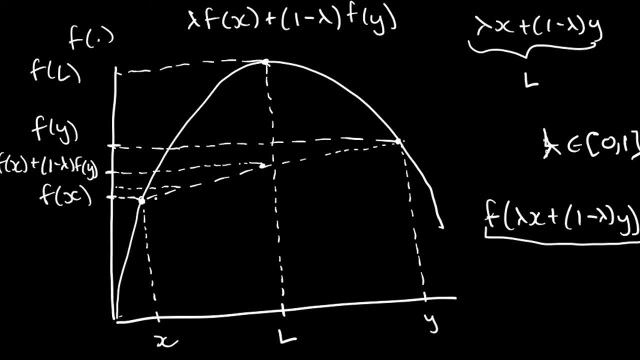 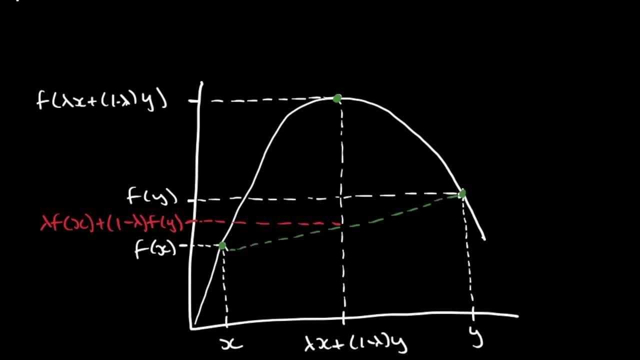 these two functions. it's going to be along somewhere on this line. As we change lambda we're going to move up or down this line. So I've just drawn this graph again, hopefully a little bit clearer, because I realized that was probably quite a lot to take in. 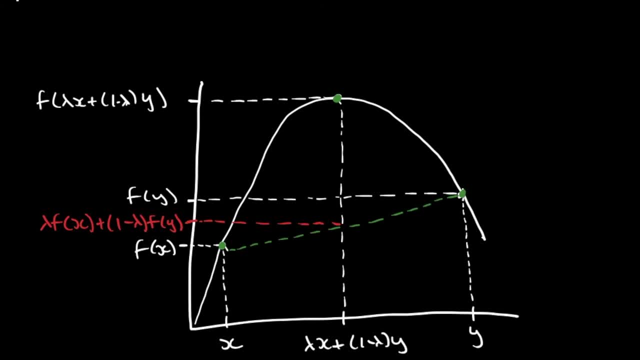 So I'm just going to go over it one more time now. Here is our linear combination of the two points and here is our linear combination of the two functions, And here is a line that is going to tell us: this is kind of the line of the linear combination. 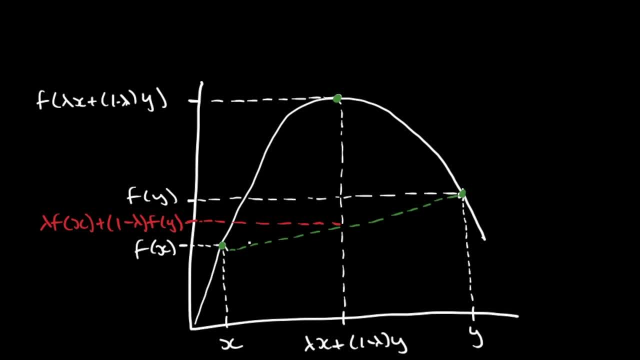 of the functions. So, as I just said, as we change lambda, we'll move up or down this line, and this line always has to be in between. Okay, So this is going to be our two points, because this is what we're taking: the linear combination. 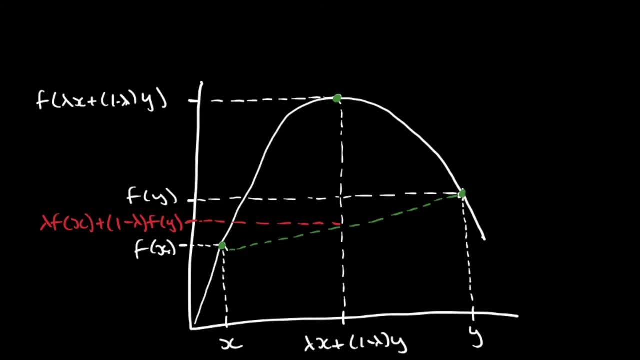 of the two points, f of y and f of x. As we can see, it's a straight line and that's why it's called a linear combination in the first place, because it's linear. So this particular function, if you haven't realized by now, just by the shape of it, this, 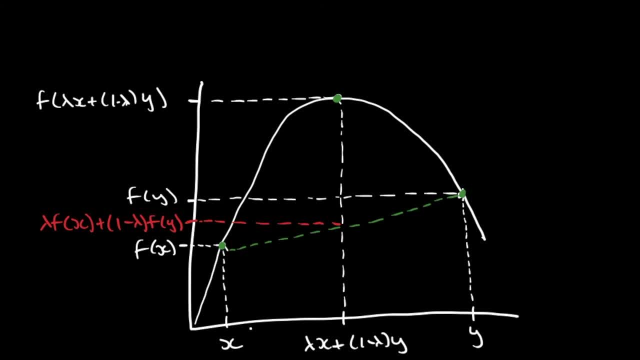 is a concave function, It's all good and well, And knowing that just by looking at it it's concave because it's got that kind of curved shape, it's got that cave like shape, We're not interested in just looking at it and being like, yes, concave, we want to actually. 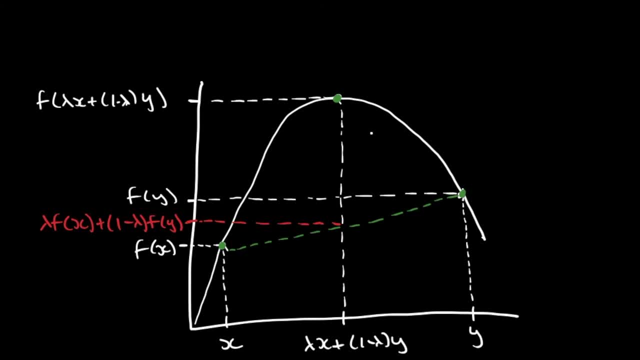 formally, mathematically, prove it with the formal definition. Because once we can actually prove that a function is concave using this kind of pretty robust definition, we can be a lot more confident the function is actually concave, instead of just looking at it and being like 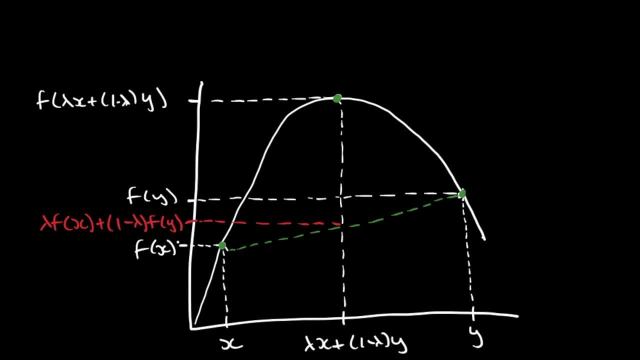 Yeah, concave. So, as we can see here, the linear combination function of linear combination is greater. This point here is greater than this point here. So in our definition of a concave function, This is what we have. So, in order to understand this a little bit better, 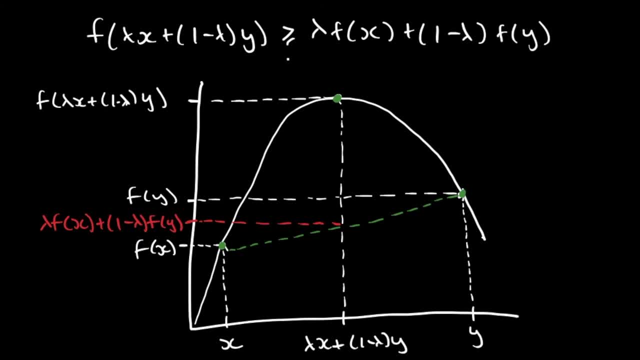 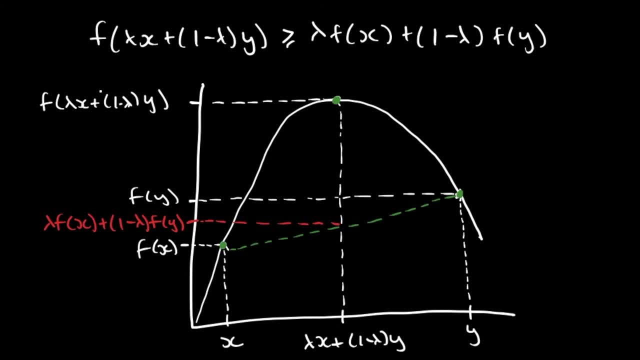 We can kind of test this. we can put this definition through some tests to see if it holds up. So let's kind of put this definition that we went through over at the beginning- that I said was the definition of a concave function- Let's put it through some tests using our example that I've drawn below. 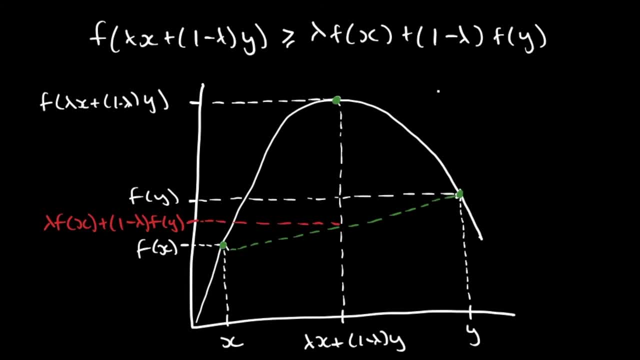 So let's kind of test this out by picking different types of lambda. So let's look at the very extreme end, for example, where lambda is equal to 1 or 0.. If lambda is equal to 0, looking at our linear combination here, we'd have the x cancel out. 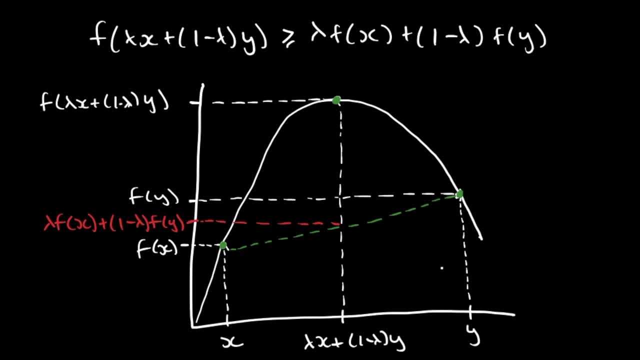 and we would have just 1 multiplied by y. So if lambda was equal to 0, our linear combination would just be here, wouldn't it be equal to 0. Where y is right now. Likewise, if lambda was equal to 1, our linear combination would be here: 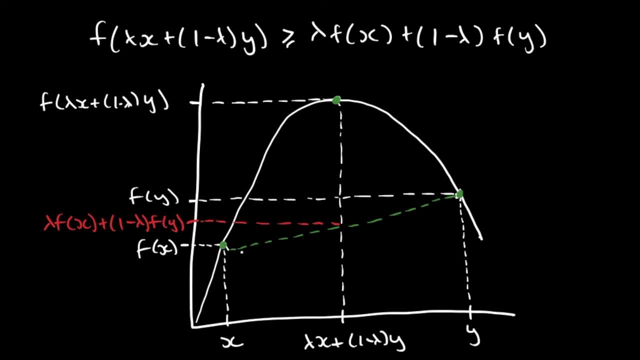 So in this case, the key point to remember is now bringing back our definition of a concave function- is that it's greater than or equal to the linear combination of the function. That's the key point, Because in this case- back again to if lambda was equal to 0, we would find a linear combination. 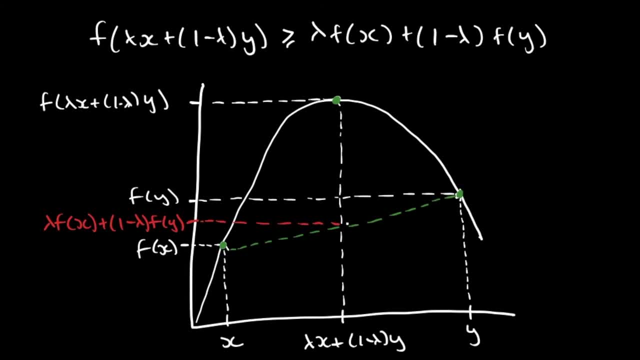 that would be equal to the linear combination of the functions, because we'd be right at the top, here in red, and we'd be again here with this. So these two would be equal to each other if lambda was equal to 0. Likewise, if lambda was equal to 1.. 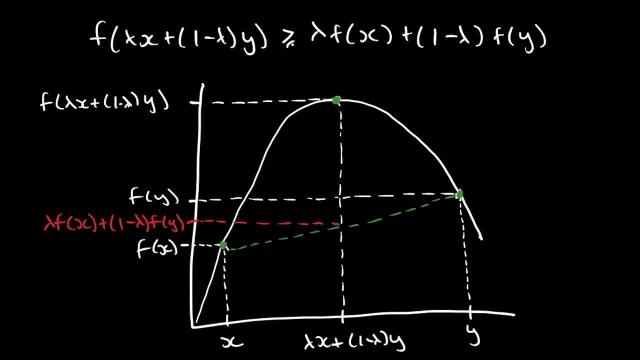 So because they can be greater than or equal to each other, this we can't. we can find any possible lambda in this example below. you can find any possible lambda and this inequality will still hold. You can try it yourself. you can try every different type of lambda, combination of lambda. 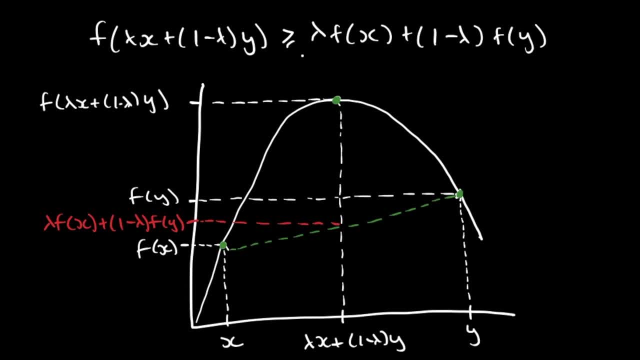 this inequality will still hold, regardless of if lambda is even on the very extreme ends of being equal to 0 or 1.. It will still hold. So we know that this is a concave function. Most of you would have already known that just by looking at the shape of it. but now 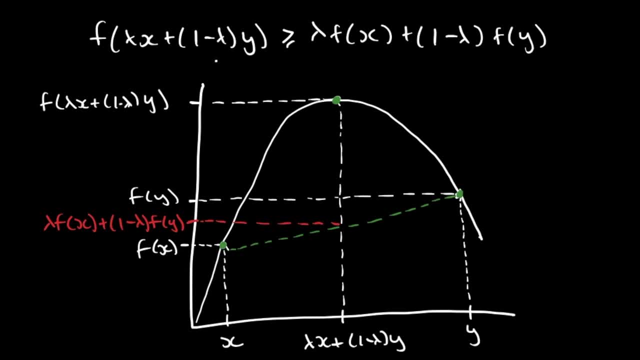 with this definition applied to it, we have proven that this is absolutely a concave function because obviously in reality, in real life, most functions are going to perfectly look nice shaped like this. So we need more of a kind of robust definition to tell us whether a function is concave or. 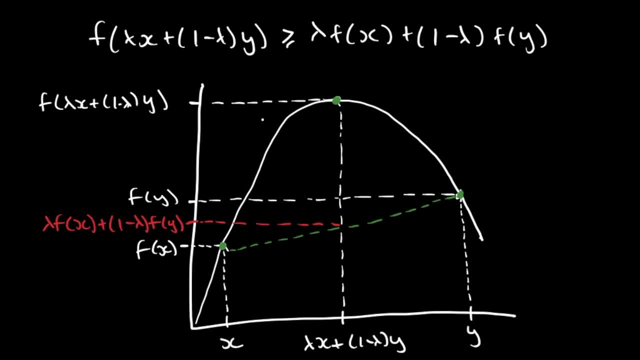 not So, rather logically, now that we've got this definition of a concave function that I mentioned at the very beginning and now I've brought it back and I've applied it to this example that we've looked at, When you look at a convex function, it is the opposite of this. 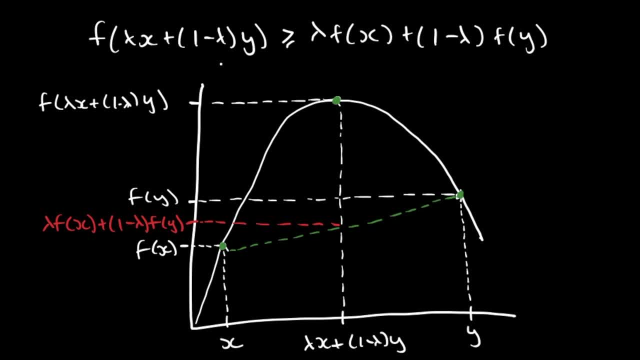 So it would be the exact same. every element here would be identical, except the inequality would be the other way. So it would look like this: It would be less than or equal to the linear combination of the functions, because in a convex function, as most of you know, rather than having this kind of cave like shape, where 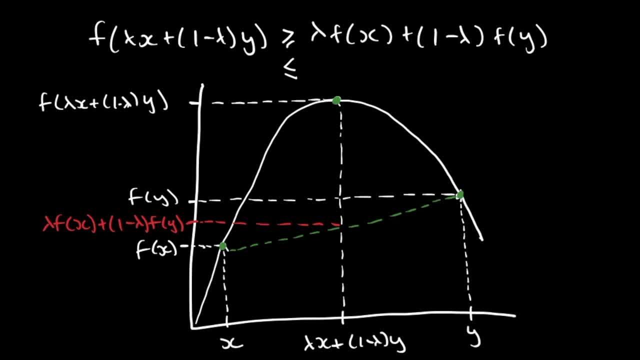 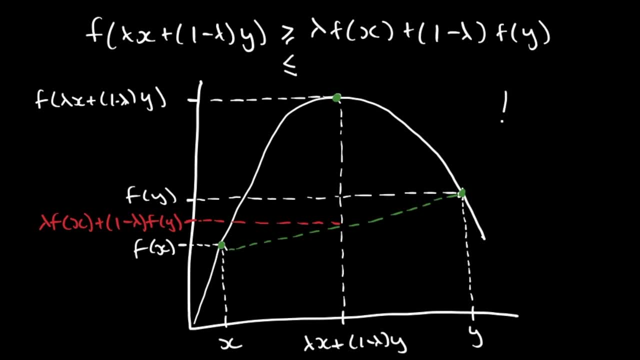 it's kind of a curve. it's got the opposite. where it kind of has a U shape, It goes up. If we were to kind of draw it on a little mini graph over here, a convex function would look something kind of like this: It would be the opposite shape to this curve cave like shape. 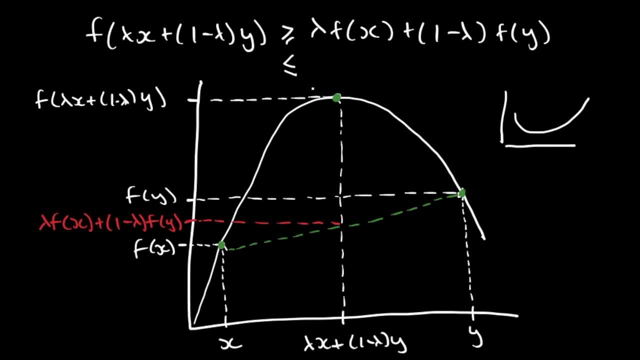 And so all we have to do is just swap the inequalities around, because we're looking at the opposite case and so you know, visually we know they're opposite ones. got this U shape one's got this cave like shape, and that kind of transfers over into this definition too. 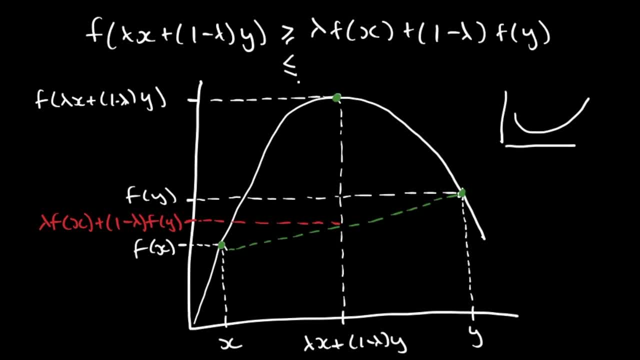 where it's just the opposite case, where we just flip the inequality around. So once you understand the convex, the concave function definition that I've kind of gone through, The, the convex function definition is pretty, pretty easy to understand because it's just the opposite case and that should be quite intuitive for you guys. 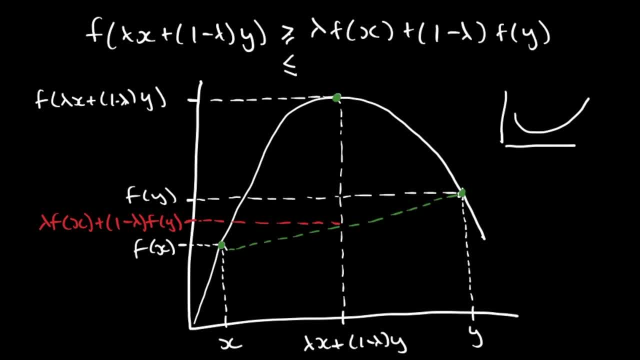 Another little side note here, because we've got greater than or equal to or less than or equal to when we would look, if we were to look at the case of a strictly concave function. Basically, You know it's in what it means: is in the definition, a strictly concave function or? 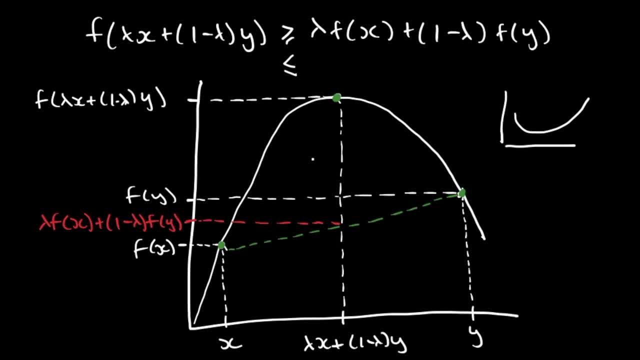 strictly convex function, which is what we didn't look at in this case. but they're just kind of small extensions of this definition, or we'd have to do is remove this. equal to so, rather than being greater than or equal to, it would just be greater than.